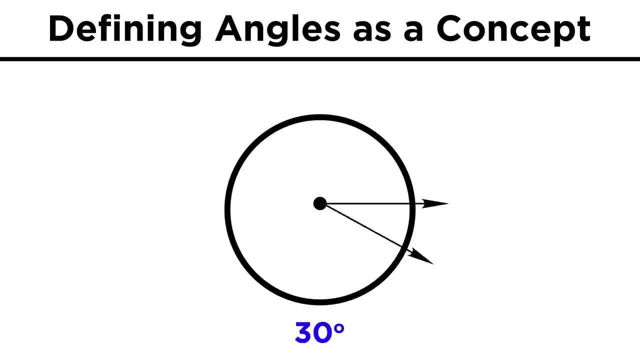 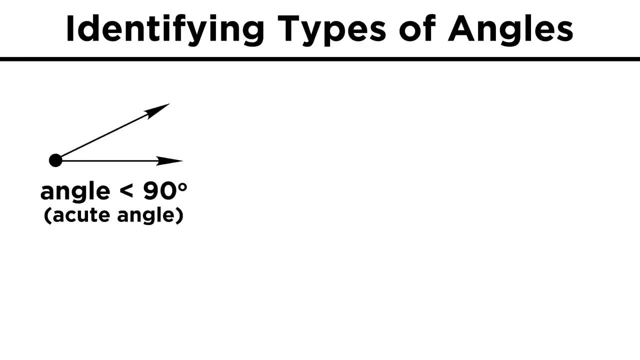 way back to zero, since the angle will be getting smaller just on the other side. Let's learn about some types of angles. If an angle is less than ninety degrees, it's called an angle of degree. If an angle is less than ninety degrees, it's called an angle of degree. 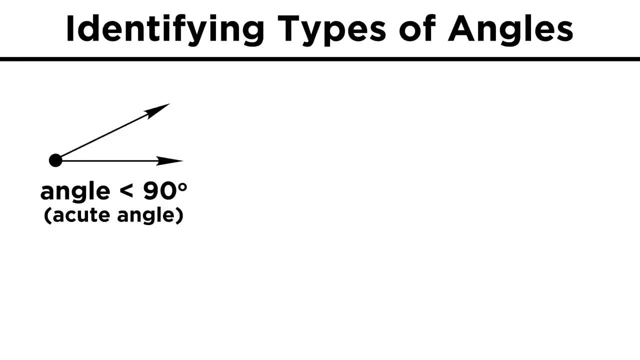 If an angle is less than ninety degrees, it's called an acute angle. We can remember this because an acute angle is cute and tiny. If an angle is exactly ninety degrees, this is a right angle and this will be denoted by a square. 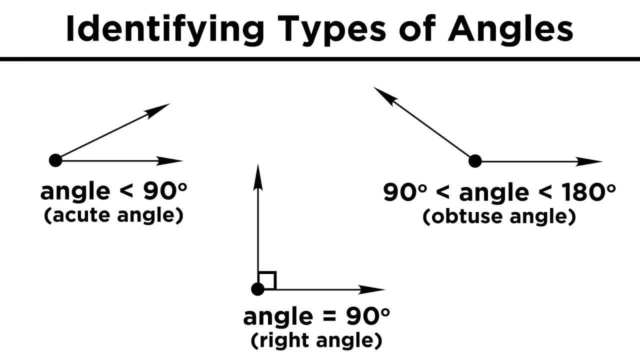 If the angle is between ninety and one hundred eighty degrees, this is called an obtuse angle, So we should now be able to look at any angle and label it as acute, right or obtuse. Now, instead of two rays, let's use two lines. 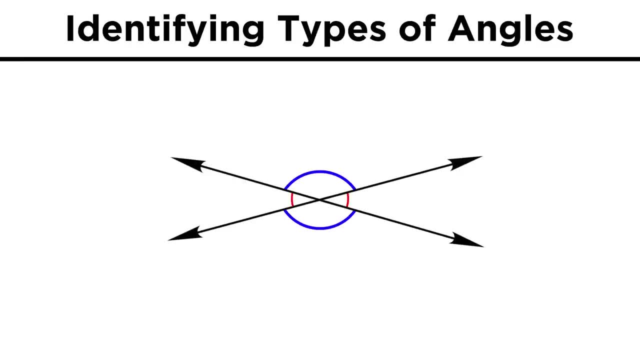 If these lines cross, we generate four angles. What are the relationships of these angles? First, we can examine the angles that are directly opposite one another, like these two. These are called vertical angles and they are always equal to one another. 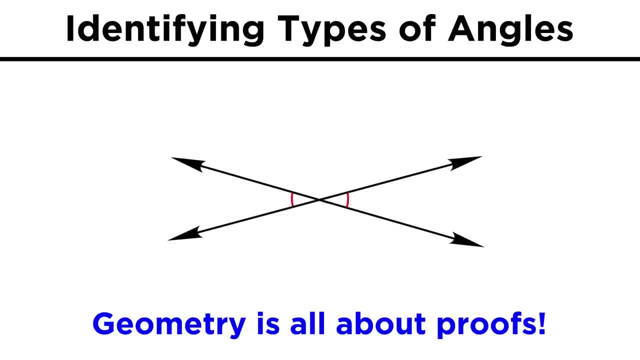 This seems intuitive by looking at the diagram, but geometry is all about rigorously proving things. that might seem obvious, though we don't know why. We can also use a vertical angle, which is called a vertical angle. We can also use a vertical angle, which is called a vertical angle. 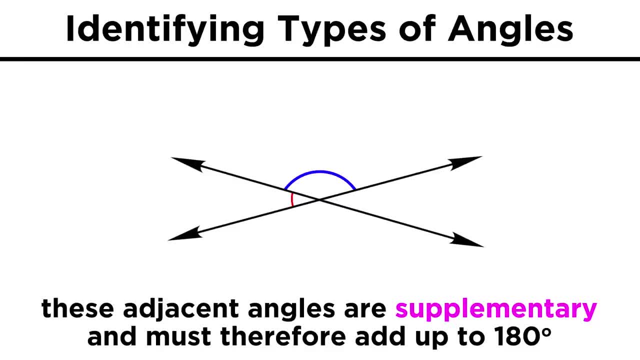 We can also use a vertical angle, which is called a vertical angle. We also have adjacent angles, which are the ones that are next to each other, and if these are the result of two lines crossing like this, these are also called supplementary. 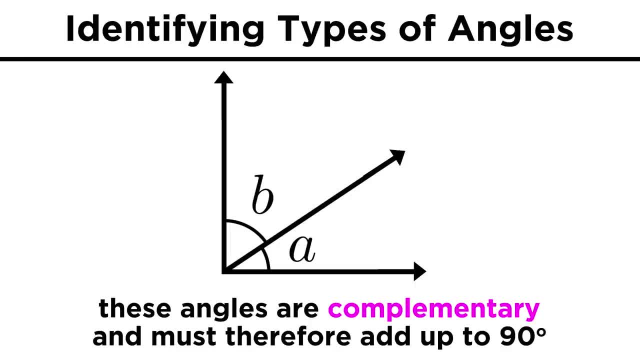 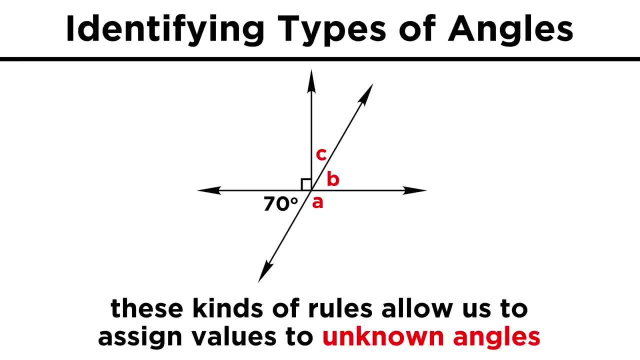 We can also have complementary angles which add up to ninety degrees. With these rules alone, we should be able to look at a diagram like this with some unknown angles and solve for the unknown angles on the basis of these rules. Let's also recall some relationships between lines. 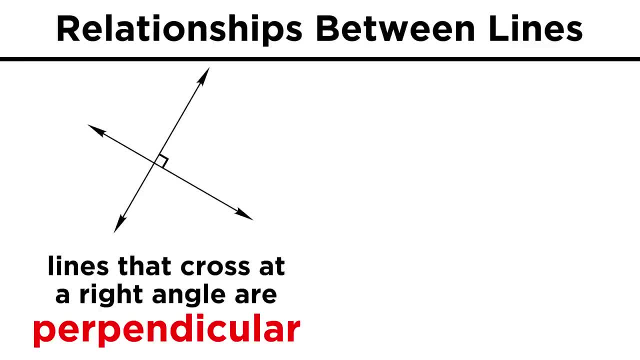 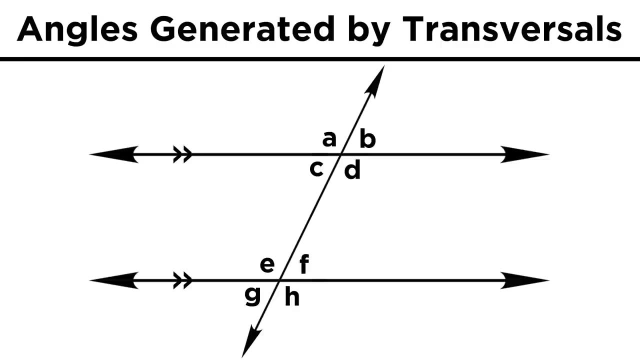 If two lines within a plane intersect at a right angle, they are called perpendicular lines. If two lines within a plane do not intersect, they are called parallel lines. If we draw two parallel lines and then a third line that crosses both of them, we can. 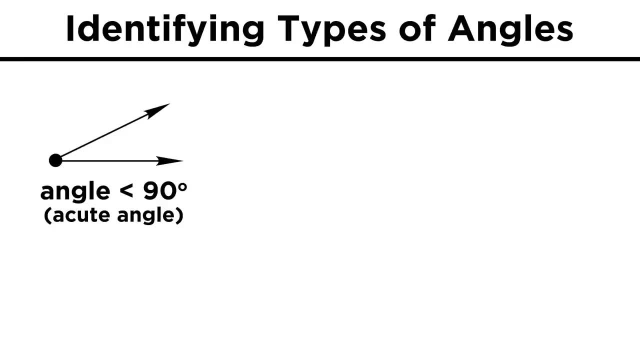 We can remember this because an acute angle is cute and tiny. If an angle is exactly 90 degrees, this is a right angle, and this will be denoted by a square. If the angle is between 90 and 180 degrees, this is called an obtuse angle. 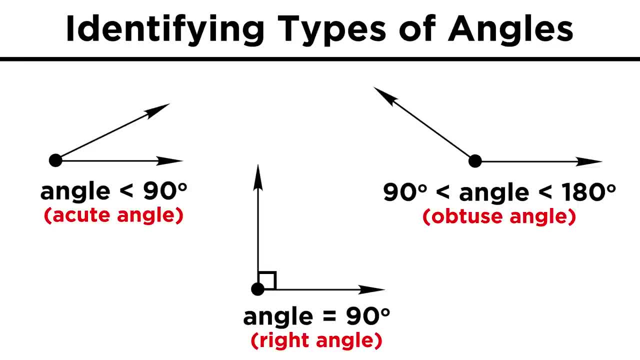 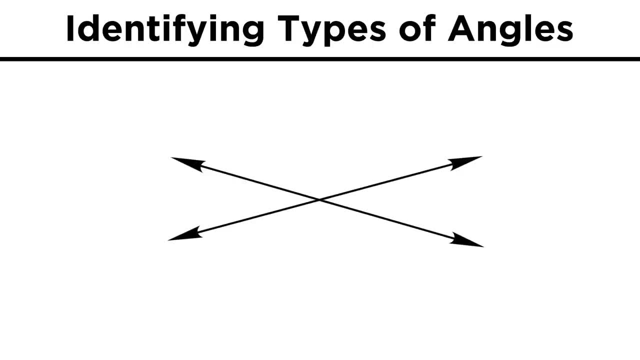 So we should now be able to look at any angle and label it as acute, right or obtuse. Okay Now, instead of two rays, let's use two lines. If these lines cross, we generate four angles. What are the relationships of these angles? 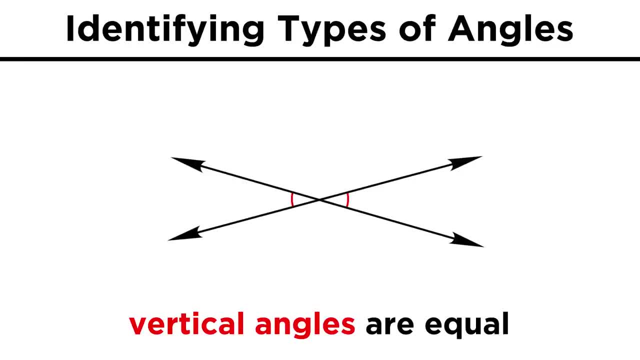 First, we can examine the angles that are directly opposite one another, like these two. These are called vertical angles, and they are always equal to one another. This seems intuitive by looking at the diagram, but geometry is all about rigorously proving things that might seem odd. 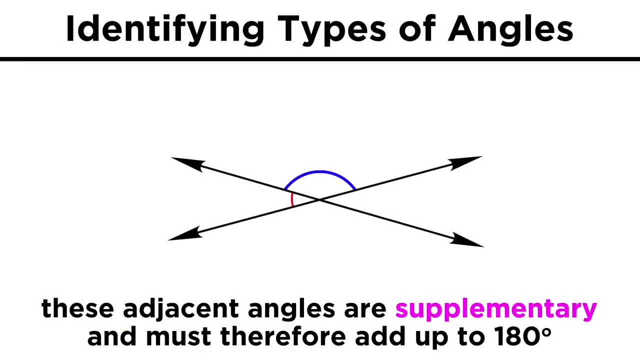 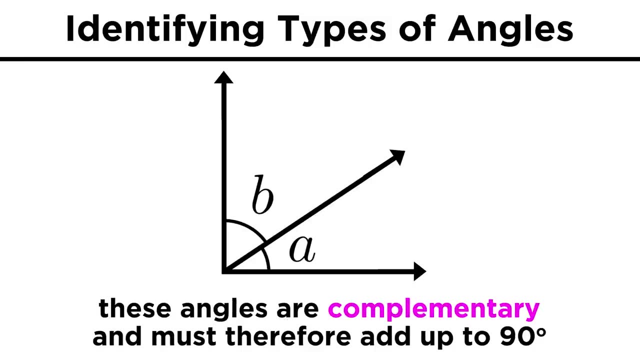 It might seem obvious, though we don't know why. We also have adjacent angles, which are the ones that are next to each other, and if these are the result of two lines crossing like this, these are also called supplementary. We can also have complementary angles which add up to 90 degrees. 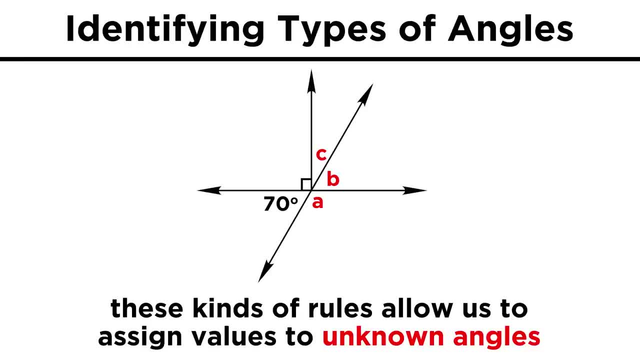 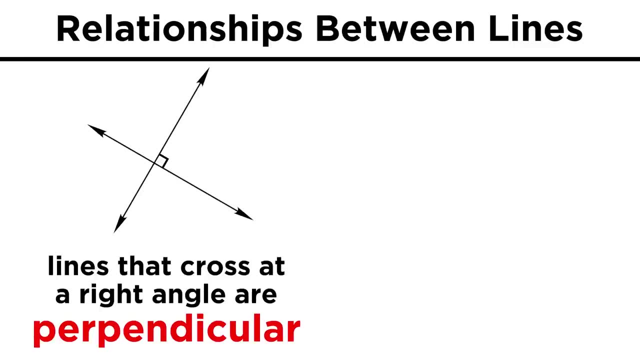 With these rules alone, we should be able to look at a diagram like this with some unknown angles And solve this problem. Solve for the unknown angles on the basis of these rules. Let's also recall some relationships between lines. If two lines within a plane intersect at a right angle, they are called perpendicular. 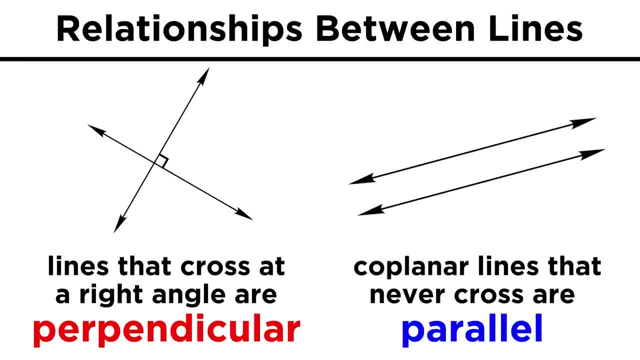 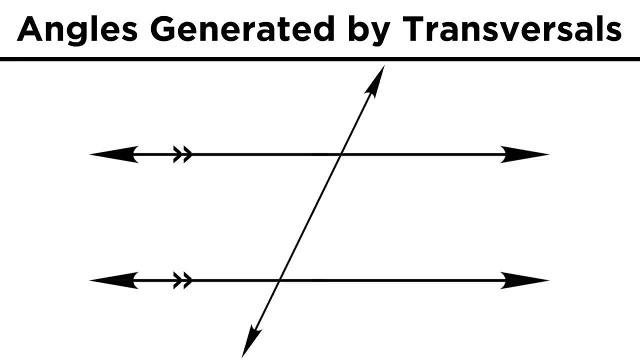 lines. If two lines within a plane do not intersect, they are called parallel lines. If we draw two parallel lines and then a third line that crosses both of them, we can define some more terms. These four angles on the inside are called interior angles. 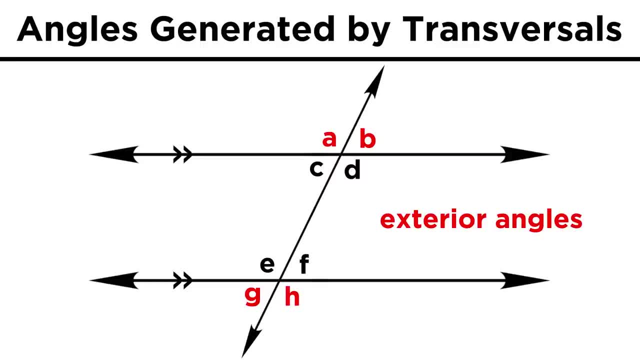 These four angles on the outside are called exterior angles Because of the relationships between vertical angles and supplemental angles. we can see that there are two sets of four equivalent angles here. First, each angle is equal to the one across from it. Then these angles here are called opposites. 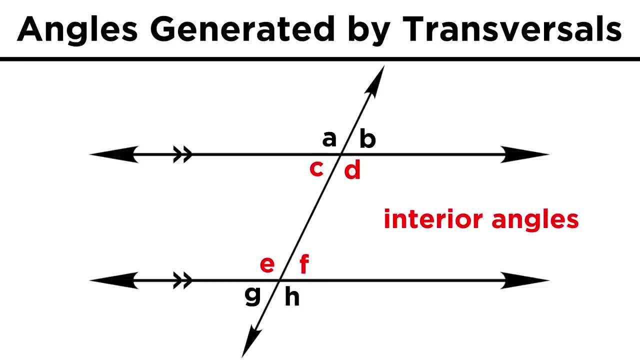 define some more terms. These four angles on the inside are called parallel angles. They are called interior angles. These four angles on the outside are called exterior angles. Because of the relationships between vertical angles and supplemental angles, we can see that there are two sets of four equivalent angles here. 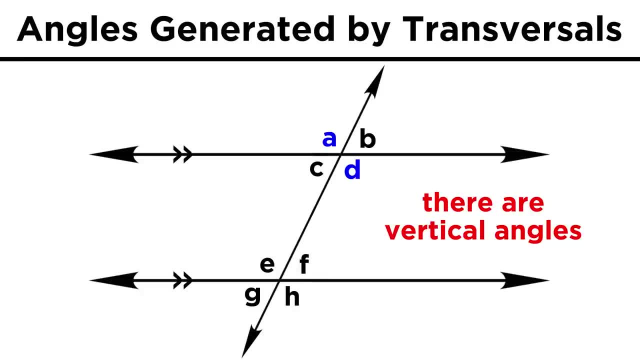 First, each angle is equal to the one across from it. Then these angles here are called alternate interior angles, and if these lines intersect they must be equal. The same goes for these alternate exterior angles. They must also be equal. This is stated by the alternate interior angles theorem and the alternate exterior angles. 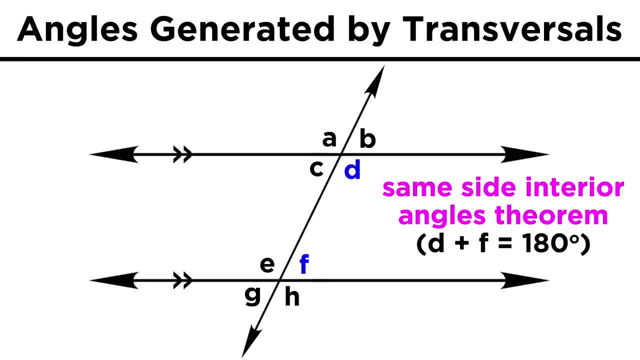 theorem. There is also the same side interior angles theorem, which tells us that interior angles on the same side of the transversal are supplementary. That makes sense, because these are supplementary And this one is equal to this one, so these two must also add up to one-eighty. 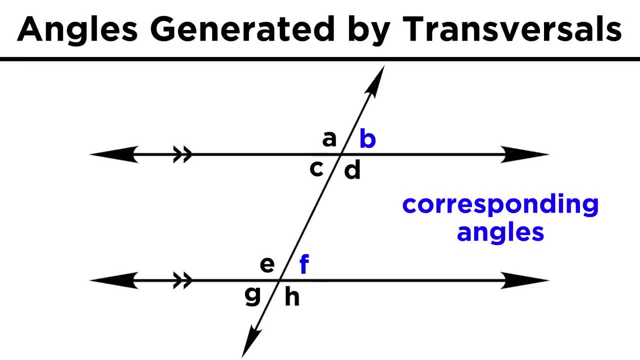 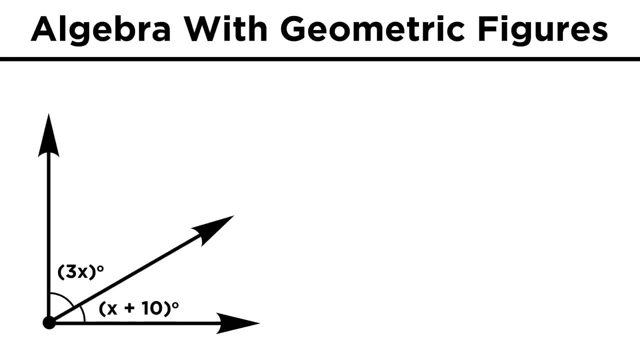 Lastly, angles in the same position with respect to one another are called corresponding angles. We will see diagrams like this quite a lot in geometry and we may even have to do algebra with them, Like if we set these complementary angles equal to three, X and X plus ten. 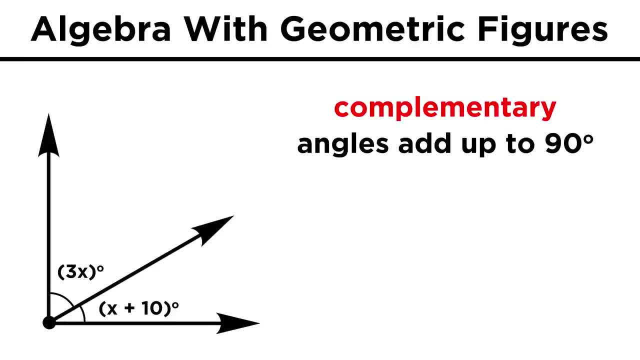 How do we find the measure of these angles? We just use the definition of the equation, The definition of complementary angles. They must add up to ninety degrees. so we make an equation, combine like terms to get four. X plus ten equals ninety, subtract ten and divide by four, which gives us twenty. 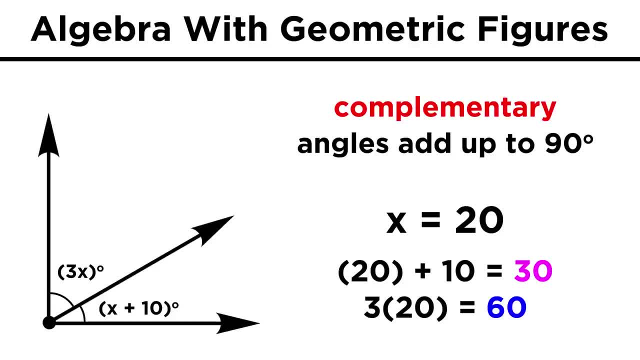 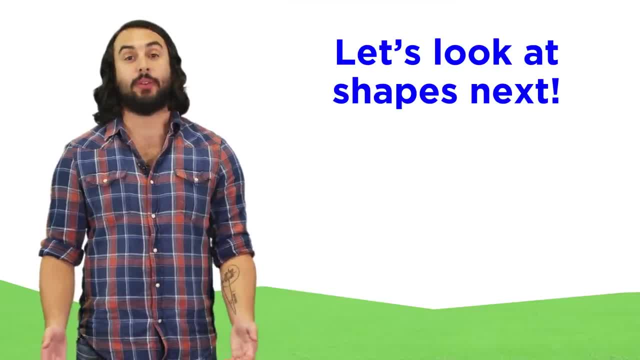 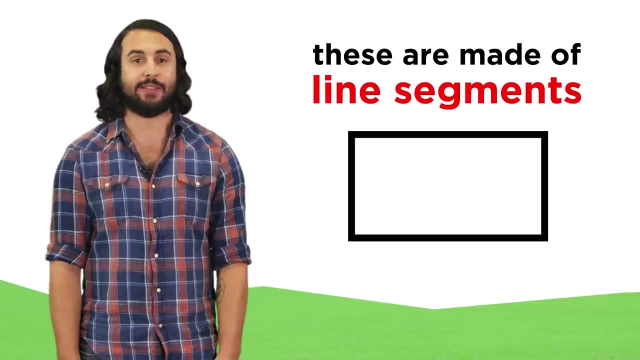 degrees for X. Plugging in twenty, that makes the angles thirty and sixty degrees. Now that we've worked a bit with lines, it's time to look at shapes, which each have some number of line segments for sides. If we are talking about straight lines, we can't have a shape with one line segment. 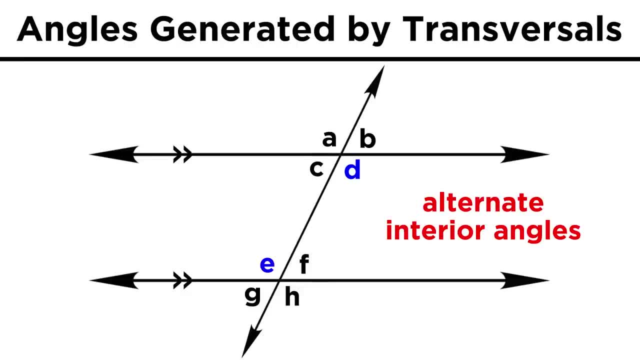 They are called alternate interior angles, and if these lines are parallel, they must be equal. The same goes for these alternate exterior angles. They must also be equal. This is stated by the alternate interior angles theorem and the alternate exterior angles theorem. 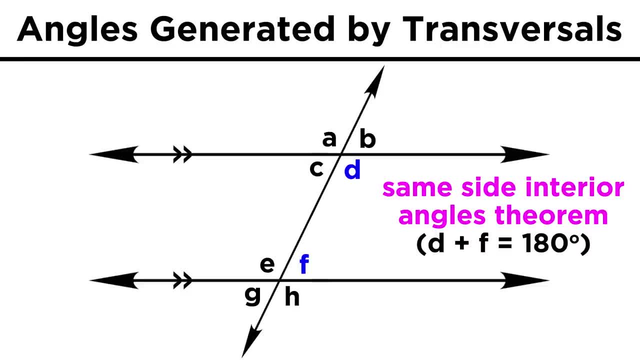 There is also the same side interior angles theorem, which tells us that interior angles on the same side of the transversal are supplementary. That makes sense, because these are supplementary and this one is equal to this one, so these two must also add up to one. eighty: 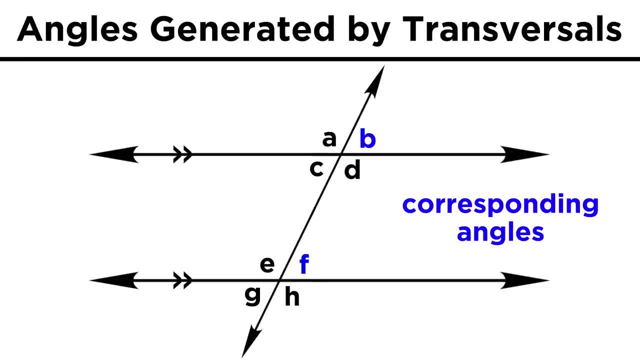 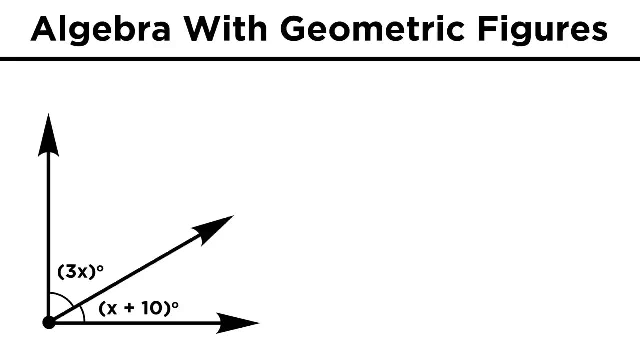 Lastly, angles in the same position with respect to one another are called corresponding angles. We will see diagrams like this quite a lot in geometry and we may even have to do algebra with them, Like if we set these complementary angles equal to three, X and X plus ten. 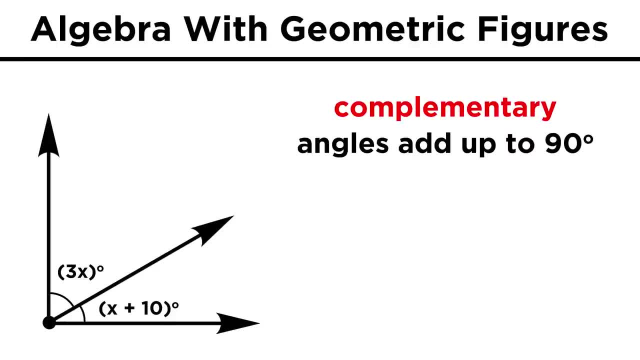 How do we find the measure of these angles? We just use the definition of complementary angles. They must add up to ninety degrees. so we make an equation. combine like terms to get four. X plus ten equals ninety. subtract ten and divide by four, which gives us twenty. 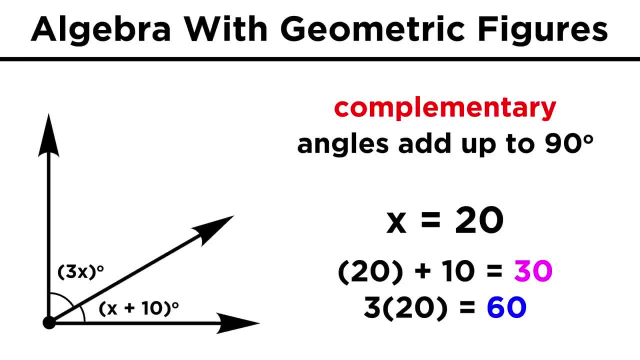 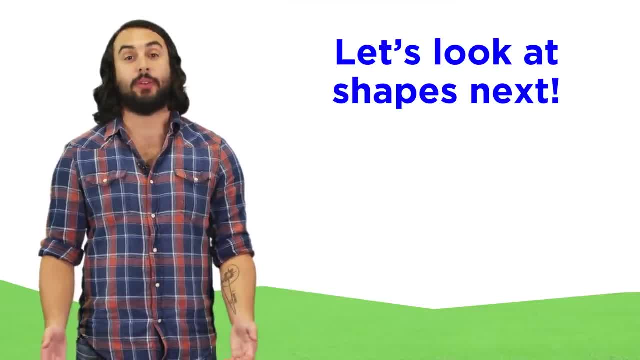 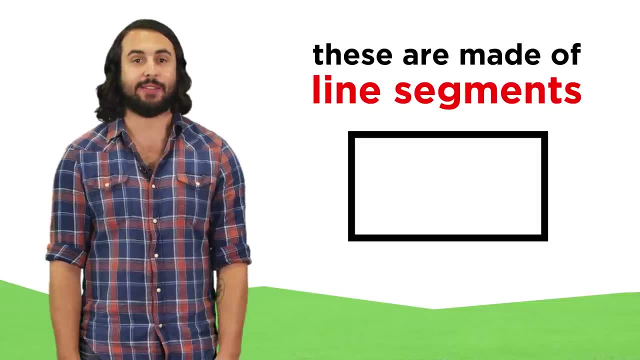 degrees for X. Plugging in twenty, that makes the angles thirty and sixty degrees. With straight lines, it's time to look at shapes, which each have some number of line segments for sides. If we are talking about straight lines, we can't have a shape with one line segment. 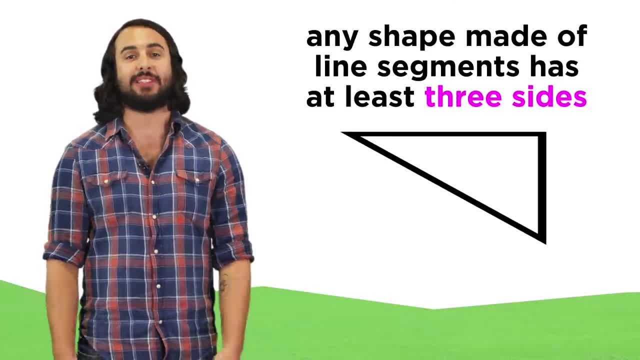 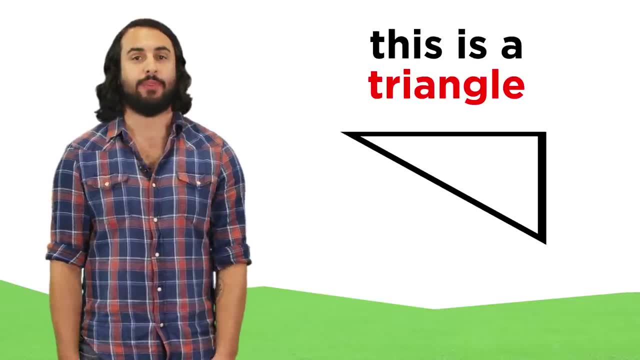 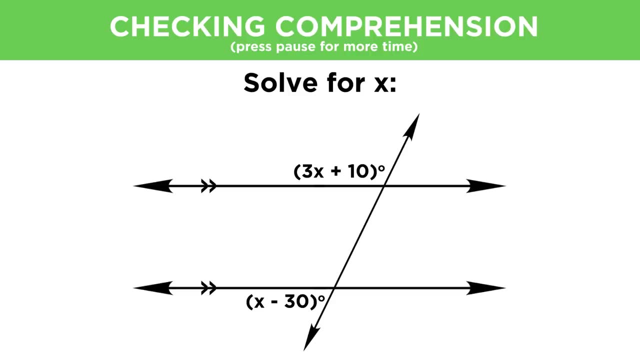 nor two. so it would seem that three line segments are the minimum required to produce a shape, and this simplest shape is called a triangle. Let's move forward and learn about all different kinds of triangles, but first let's check the inside out. 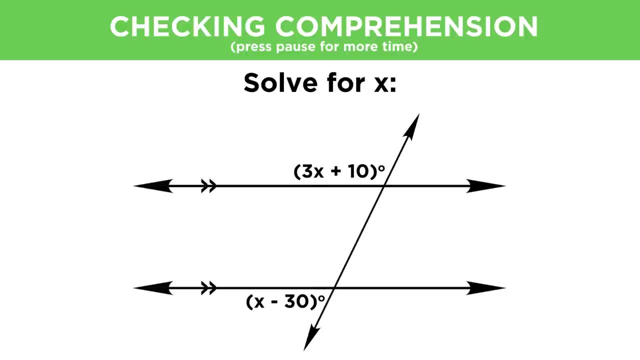 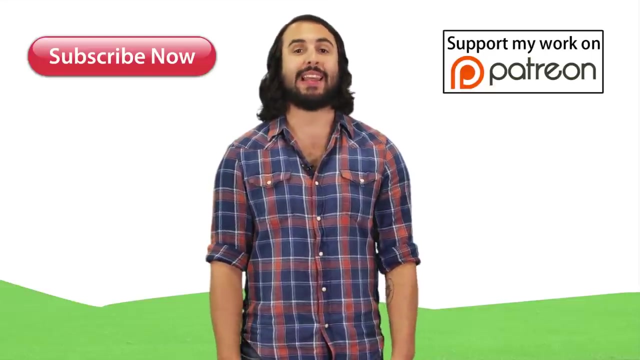 Yarn Overhead- Sideways, Sideways, Sideways, Sideways, Sideways, Sideways, Sideways. Thanks for watching, guys. Subscribe to my channel for more tutorials. support me on patreon so I can keep making content and, as always, feel free to email me professordaveexplains at gmail dot com.